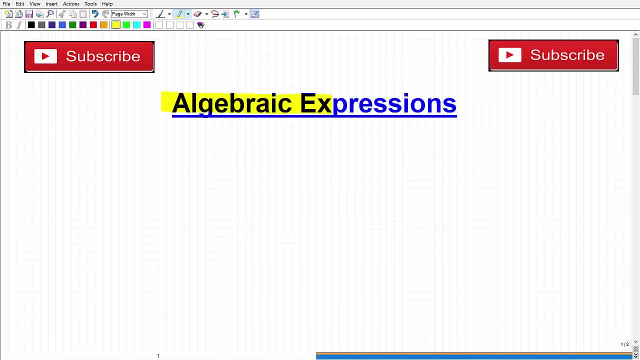 Okay, algebraic expressions. I'm going to teach you everything you need to know as an algebra student or whatever math level you're taking. I'm going to teach you all the fundamental things about algebraic expressions, and it's pretty simple. So that's just ahead Before we get started. if you're new to my YouTube channel, I literally have hundreds of videos that I think you'll find very helpful, So I hope you consider becoming a subscriber And if you're looking for 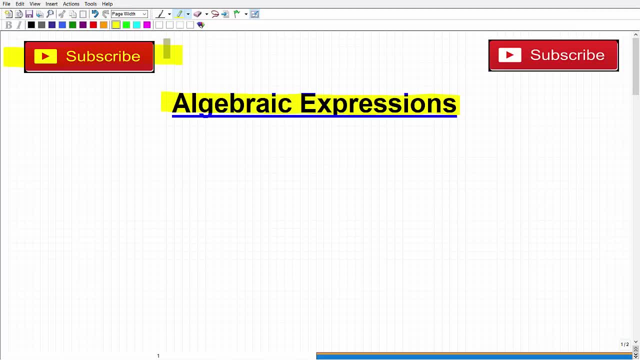 you know, additional really comprehensive, step by step instruction. I have a math academy. I'll leave a link in the description in the video if you're interested in checking out my courses. But with that being said, let's get into algebraic expressions. So let's take a look at what this means, And let's do this by looking at the two root words here. So one is algebra right And the other one here is expressions. So what does this mean? 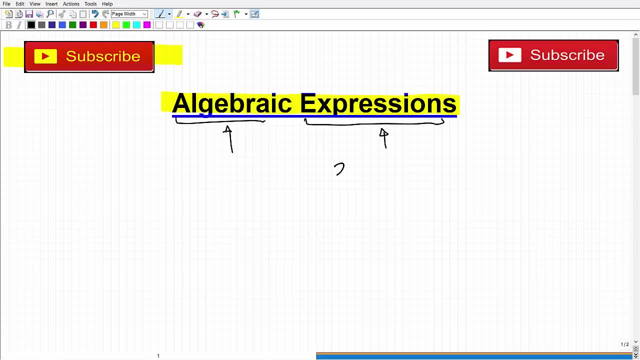 Well, let's start with the expression part first. So something like this is an example of an expression. I'm just kind of writing a few things down here, Let's see, maybe something like this: Okay, these two things are examples of expressions in mathematics. Okay, notice, I said mathematics and not algebra. Let's just keep it kind of general expressions. Now, why are they expressions? Because they're expressing something. Okay, basically, they're just making a statement, It's just 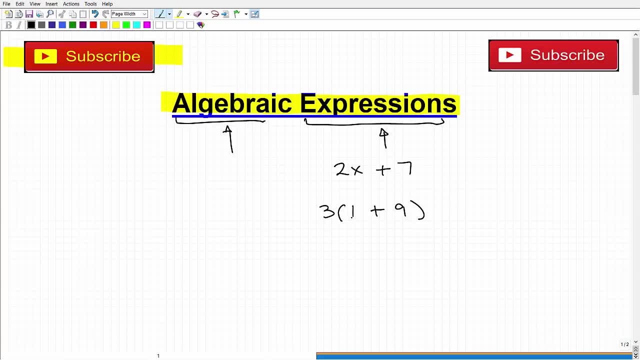 some numbers and some operations. Now this is in contrast to things that are different. Okay, what if I have an equal sign And let's say, let's put another number over here, let's say 20.. Now this right here is an equation. So if I have this, I would. I would refer to this as an a, a, an equation, And because it has a variable, this could be an algebraic equation, want to kind of give it a little bit more description. So in mathematics we have 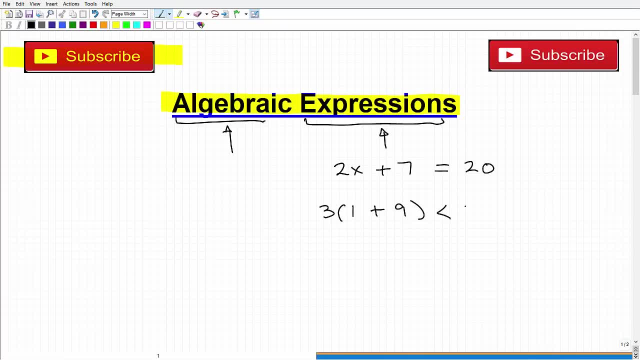 expressions and we have equations, and we have and we also have things like inequalities. okay, so if you have something with the inequality symbol, that you would refer to that as an inequality, not an equation. or an expression with an equal sign, okay, that's an equation, not an expression. and then if you just have something, all by, 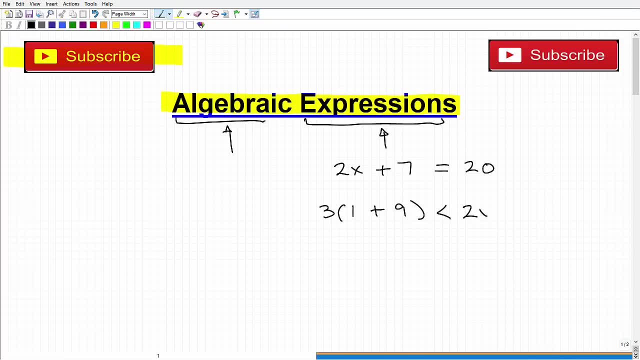 equations. So we have expressions and we have, and we also have things like inequalities. okay, so if you have something with the inequality symbol, that you would refer to that as an inequality, not an equation. or an expression with an equal sign, okay, that's an equation, not an expression. and then if you just have something, all by, 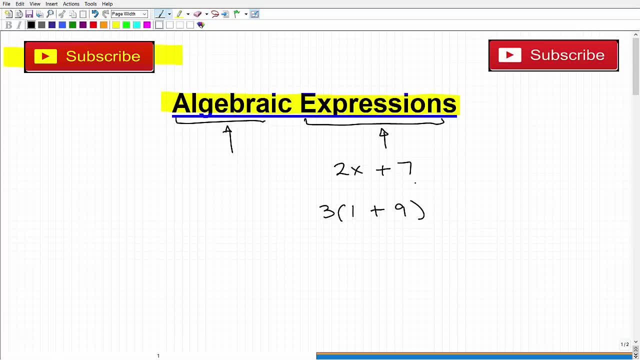 itself like: so these are just expressions. okay, now of course I'm going to get into and what an algebraic expression is, but let's, let's, let's first just start with a numeric expression. so we have algebraic expressions and we have numeric expressions. so right here, this is an. 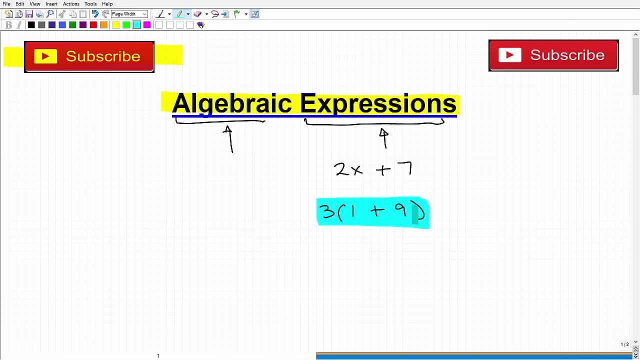 example of a numeric expression. why? because it just involves numbers. okay, as soon as you have a variable thrown into the mix, you have an algebraic expression. so this is a very basic definition of what an algebraic expression is, and it's what an algebraic expression is. but let's look at another numeric expression. 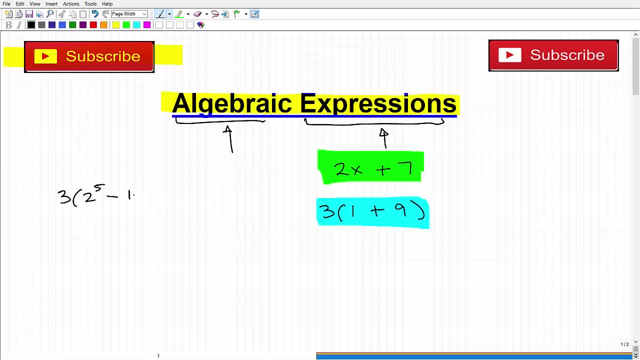 okay, let's, let's know, I'm just gonna make something up here. so this right here will be referred to as a numeric expression. and in order to simplify this numeric expression, we need what the order of operations correct. so all this ties in, so I can give you a, a promise: a simplified and numeric. expression, so I can give you a a problem. I say: simplify the numeric expression, so I can give you a a problem. I say: simplify the numeric expression, so I can give you a a problem. I say: simplify the numeric expression, so I can give you a problem. I say: simplify the numeric expression, so I can give you a a problem. 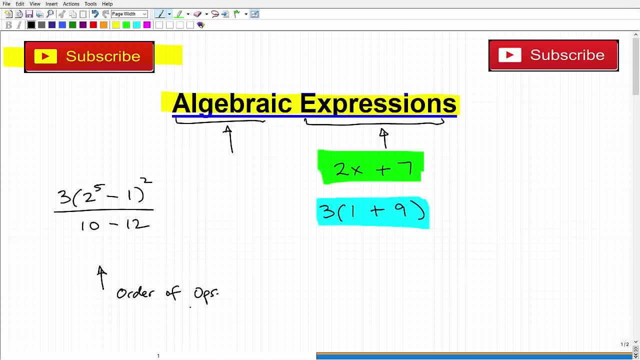 you say, okay, after all these calculations. so I'm gonna use the order of operations. so pretty much kind of you know the same approach when we're talking about algebra, but there are going to be some, some things that are specific to algebra and algebra fundamentals, and I'm gonna get into that. 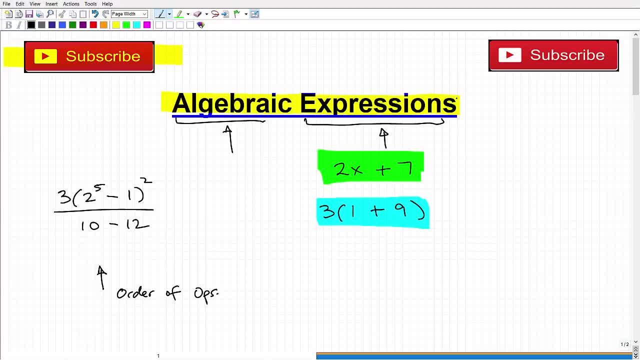 next. okay, so first things first. I wanted you to understand what the word expressions are in mathematics in general. okay, so we have numeric expressions and we have algebraic expressions. okay, now let's, let's go ahead and take this a step further. and our algebraic expressions: so 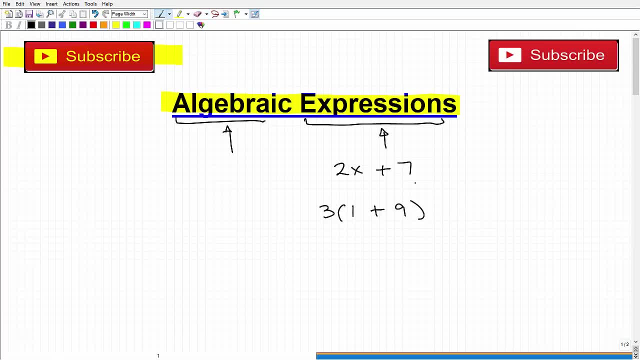 itself like: so these are just expressions. okay, now of course I'm going to getting into and what an algebraic expression is, but let's, let's first just start with a numeric expression. so we have algebraic expressions and we have numeric expressions. so right here this is an example of a numeric. 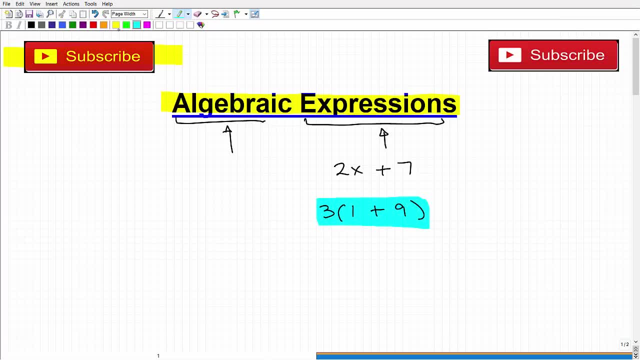 expression? why? because it just involves numbers. okay, soon as you have a variable thrown into the mix, you have an algebraic expression. so this is a very basic definition of, For short, A ultraclass football team. an algebraic expression is. but let's look at another numeric expression. okay, 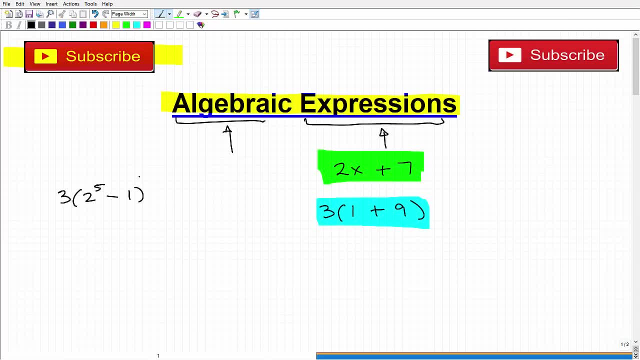 let's, let's. I'm just gonna make something up here. so this right here would refer to as a numeric expression. and in order to simplify this numeric expression, we need what the order of operations correct. so all this ties in, so I can give you a problem. I say: simplify the numeric expressions. you say: 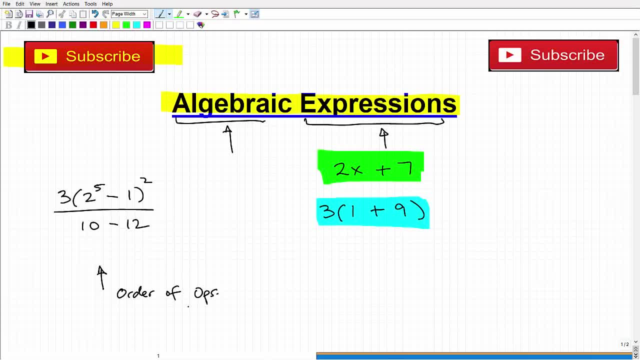 okay, I have to do all these calculations, so I'm going to use the order of operations, so pretty much, kind of you know, the same approach when we're talking about algebra, but there are going to be some, some things that are specific to algebra and algebra fundamentals, and I'm gonna get into that. 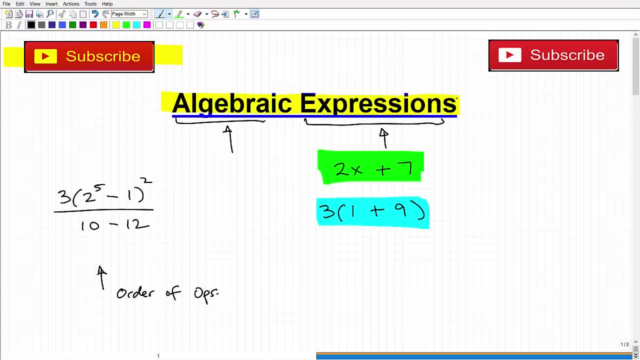 next. okay, so first things first. I wanted you to understand what the word expressions are in mathematics in general. okay, so we have numeric expressions and we have algebraic expressions. okay, now let's go ahead and take this a step further. and our algebraic expressions? so let's take. 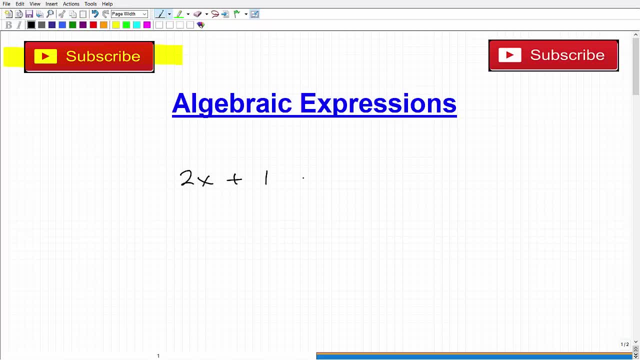 something like this, just making things up here, all right. so often times when you're just starting to learn algebra, you're given algebraic expressions and what they mean is they can be in three different languages and they're labeled in by one or two different languages. and I'm gonna give you some examples of the. 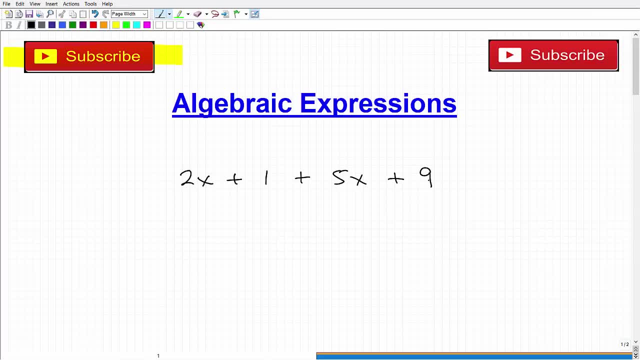 expressions. we have numeric expressions and we have algebraic expressions. okay, now What your teacher wants you to know is how to simplify algebraic expressions. So this is one of the things that you're going to be asked to do, So to simplify an algebraic expression. what you want to look for are combining things. 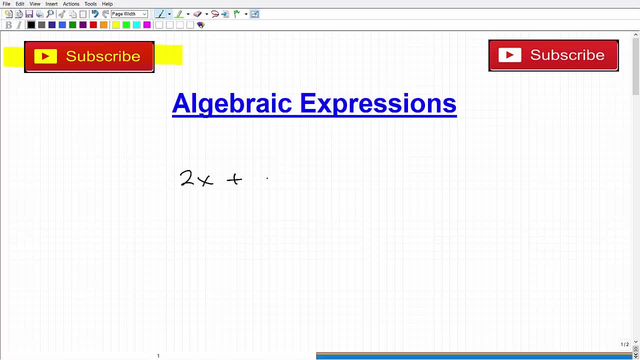 let's take something like this, just making things up here, all right. so oftentimes, when you're just starting to learn algebra, you're given algebraic expressions and what your teacher wants you to know is how to simplify algebraic expressions. so this is one of the things that you're going to be asked to do, so 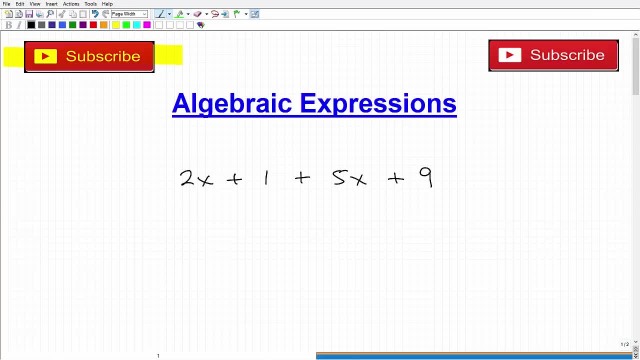 to simplify an algebraic expression. what you want to look for are combining things that are alike- okay, so things that are like. so what are like items in an algebraic expression? well, we can combine numbers, alright. so numbers, you can always add them to your algebraic expression. you can always add them to. 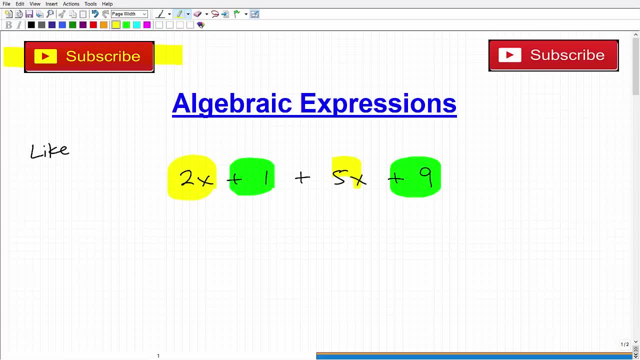 that up right. and then we have these items here, these variable components to our expressions. so each one of these guys here is called a term. okay, so we're looking at algebraic expression, the things that have variables, we we refer to them as terms. so a term? let's take a look at this term here. 2x has a couple. 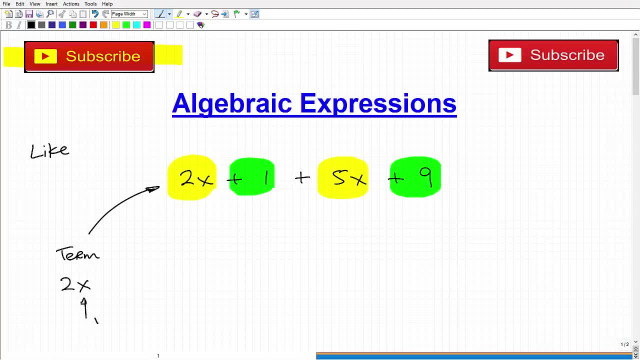 different components to it. one: it has a variable, okay, and then the number in front of the variable is referred to as a coefficient. okay, so this term here, 2x, has a coefficient of 2 and its variable is X. okay, this term here, 5x, has a coefficient of 5 and its variable is X. 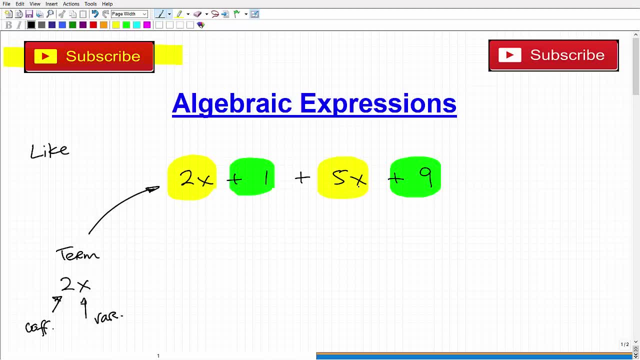 so what we're looking to do in algebraic expressions is to simplify them. okay, we want to make them as simple as possible, so we what we're going to do is combine numbers. so we're going to add these guys up here in a second and then we're going to see if we can combine these two terms. 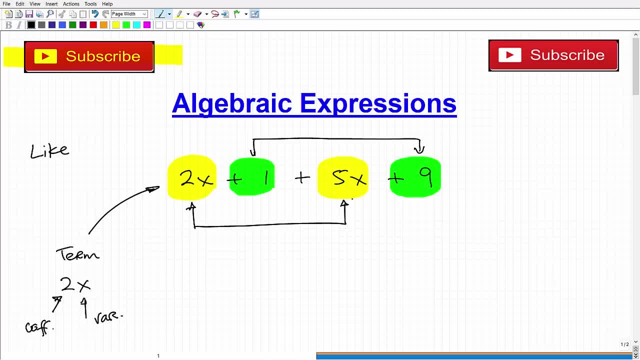 okay, we can combine two terms if they're like, alright. so we have to ask ourselves: are these like terms? okay, well, here's the key, here's how you know. if two terms are like, they're variable parts, okay, have to be exactly the same, okay. so, for example- and well, let me just say this much- in these, in this case, 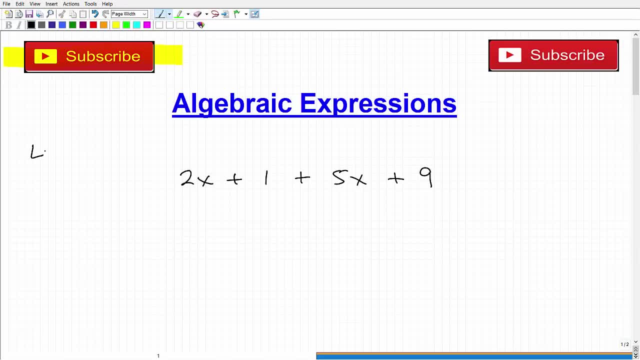 that are alike, So things that are alike. So what are like items in an algebraic expression? Well, we can combine numbers, so numbers you can always add up right. And then we have these items here, these variable components to our expressions. 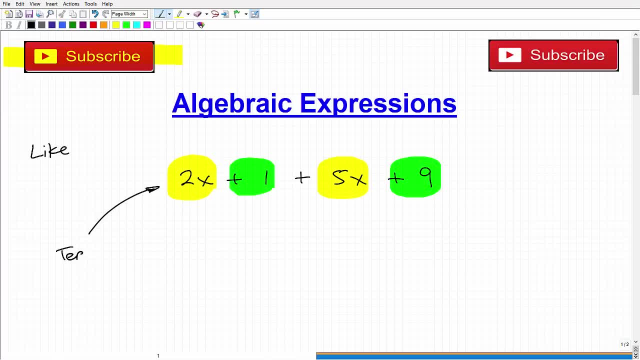 So each one of these guys here is called a term. Okay, so when we're looking at an algebraic expression, the things that have variables- we refer to them as terms. So a term- let's take a look at this term here- 2x has a couple different components. 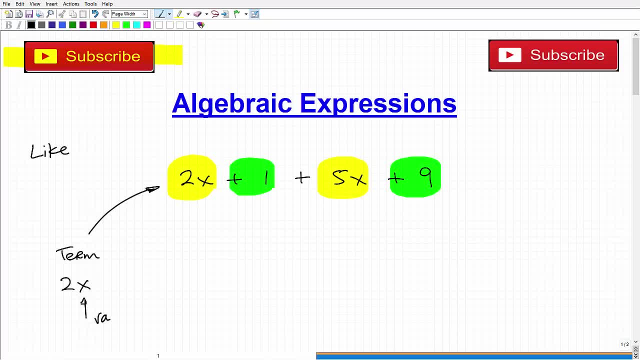 to it One: it has a variable, Okay, And then the number in front of the variable is referred to as a coefficient, okay, So this term here, 2x, has a coefficient of 2 and its variable is x. 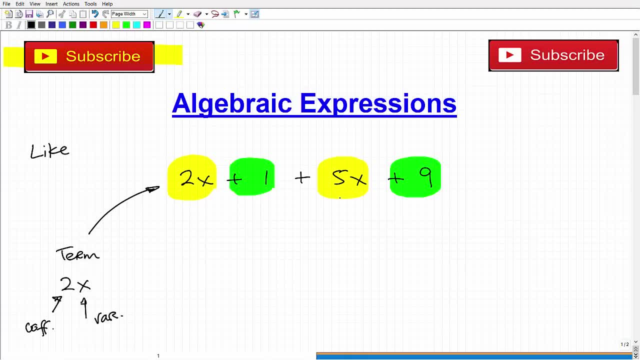 Okay, This term here, 5x, has a coefficient of 5 and its variable is x. So what we're looking to do in algebraic expressions is to simplify them. We want to make them as simple as possible, So what we're going to do is combine numbers. 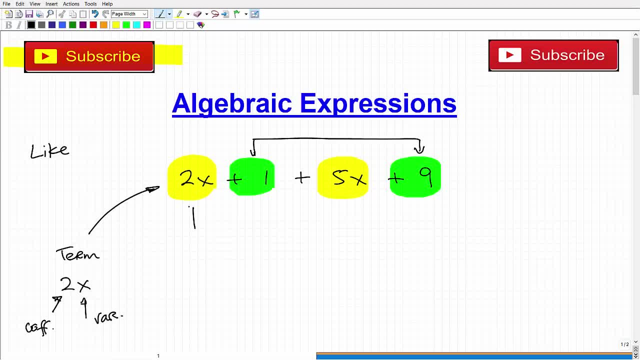 So we're going to add these guys up here in a second And then we're going to see if we can combine these two terms. okay, We can combine two terms. if they're alike, all right. So we have to ask ourselves: are these like terms? 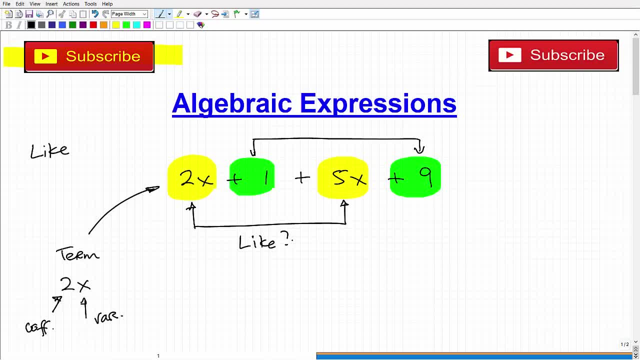 Okay. Well, here's the key. Here's how you know: if two terms are alike, Their variable parts- okay, have to be exactly the same. Okay, So, for example- well, let me just say this much: In this case, here they both have exactly an x, so we can combine them. 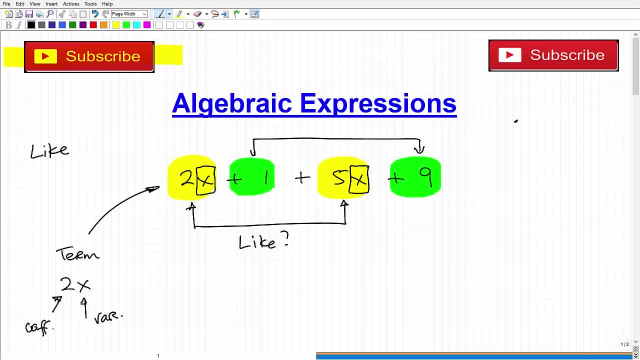 So we're going to do that here in a second. but let's take a look at something. If I have 2x and 5x- these are like terms because they have exactly the variable x- okay, But what if I have 2x and 5x squared? 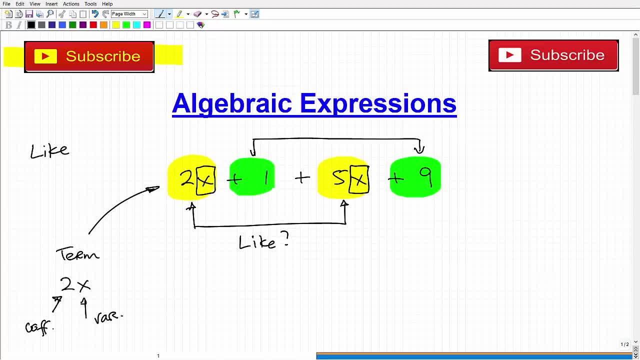 here they both have exactly an X, so we can combine them. so we're going to do that here in a second. but let's, let's take a look at something. if I have 2x and 5x, these are like terms because they have exactly the variable X. okay, but 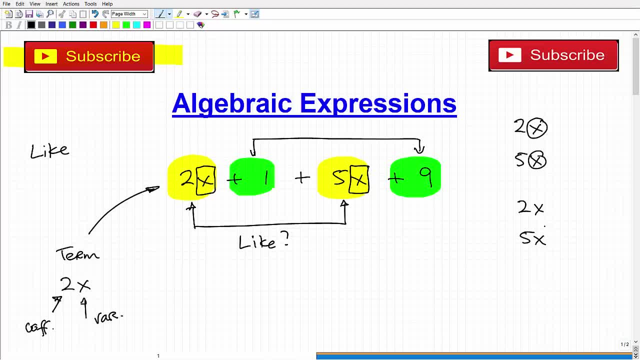 what if I have 2x and 5x squared? okay, now, they're pretty close, but this is an X squared, this is an X. so these are not like terms. okay, and these are okay. these are like like terms. okay, now the variable components can be much. 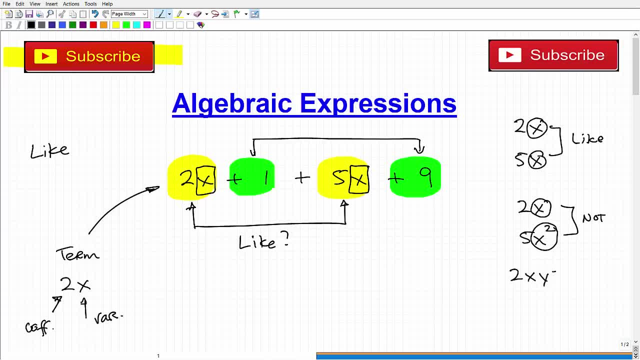 more complicated. so we can have like say 2x Y Z and 5x Y Z. so they're variable terms here. these parts are exactly the same, so we can combine them okay. and as soon as one of these are a little bit off, let's say: this is Z squared now. 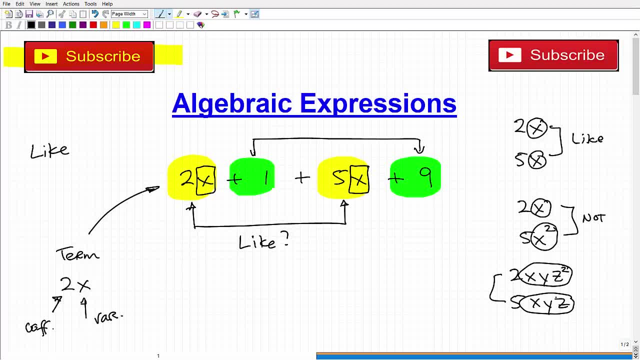 they're different. now they're, they're not like, okay. so one of the big things you need to understand about algebraic expressions is under this understanding of terms and to understand to know if terms are like or not like, okay. so again, I've done a lot more videos on like terms, if you check them there in my 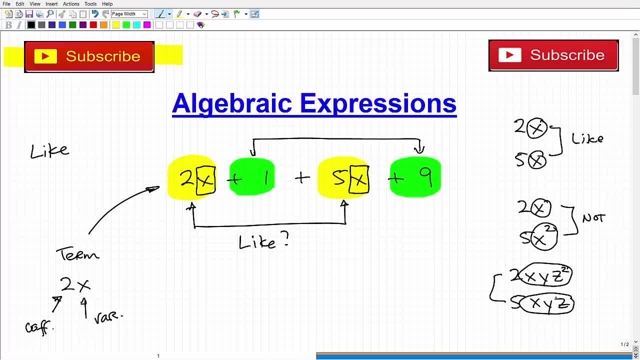 algebra playlist. so if you go to algebra and you go to algebra and you go to algebra, so you can check those out, but I think, hopefully you got the pretty basic idea. I mean, again, this stuff doesn't have to be difficult, so let's get, let's get to this problem here. all right, now let me erase this. we're not. 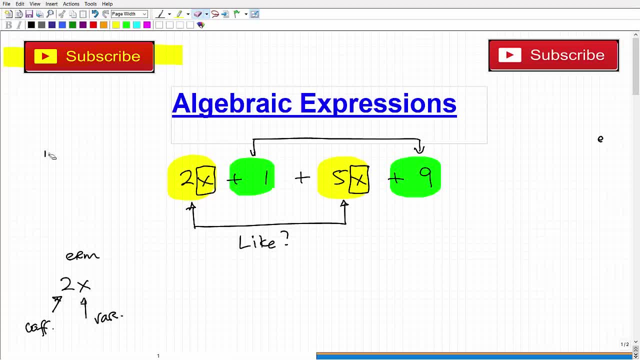 too cluttered, all right. so again, when we're talking about algebraic expressions, one of the things- one of the most common things- you're going to be asked to do is to simplify them. so we're going to look to see if there's any way we can combine, combine the components that make up the expression. 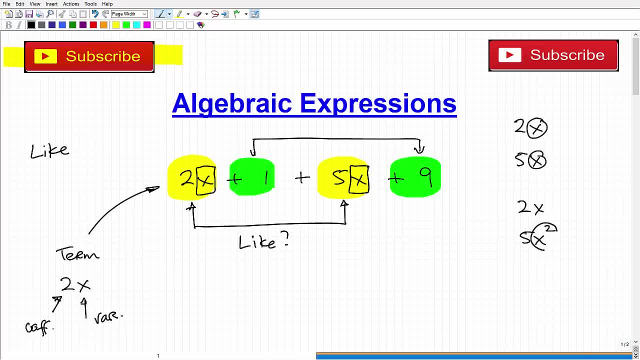 Okay, Now they're pretty close, but this is an x squared, This is an x squared, This is an x. So these are not like terms. okay, And these are okay, These are like terms okay. Now the variable components can be much more complicated, so we can have, like, say, 2xyz. 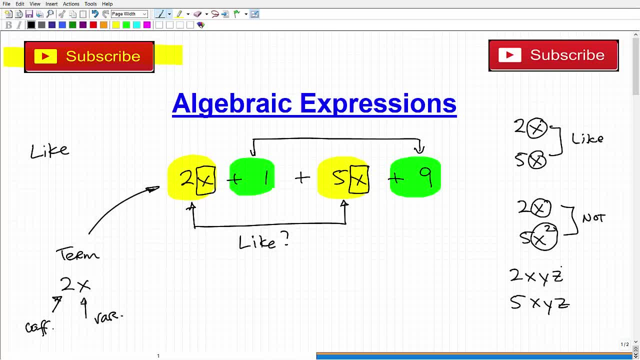 and 5xyz, So their variable terms. here. these parts are exactly the same, so we can combine them, okay. And as soon as one of these are a little bit off, let's say: this is z squared, now they're different. 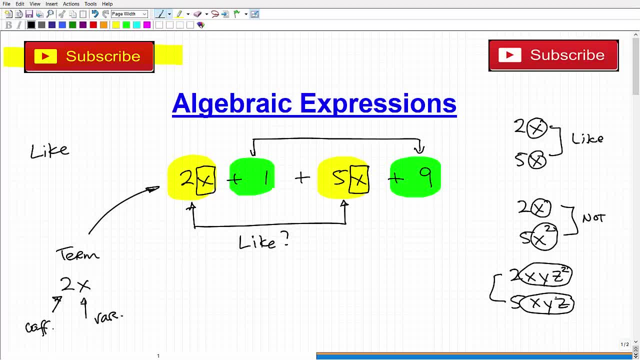 Now they're not like okay. So one of the big things you need to understand about algebraic expressions is this understanding of terms and to know if terms are like or not like okay. So again, I've done a lot more videos on like terms. if you check them, they're in my algebra. 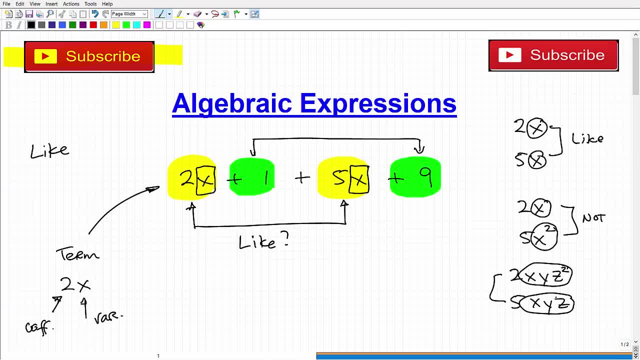 playlist. You can check those out, but I think hopefully you got the pretty basic idea Again, this stuff doesn't have to be difficult, so let's get to this problem here. all right, Now let me erase this so we're not too cluttered. 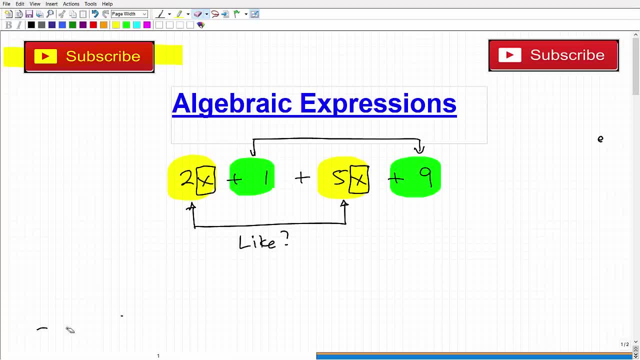 All right. so, again, when we're talking about algebraic expressions, one of the things, one of the most common things you're going to be asked to do is to simplify them. So we're going to look to see We can combine, combine the components that make up the expression. 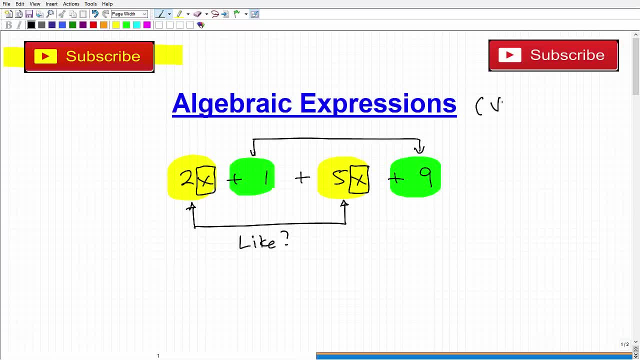 So what's going to make up an algebraic expression? are going to be variable, variable terms, right, And numbers, And these numbers can be fractions, they can be integers. positive, negative decimals doesn't make a difference, right. 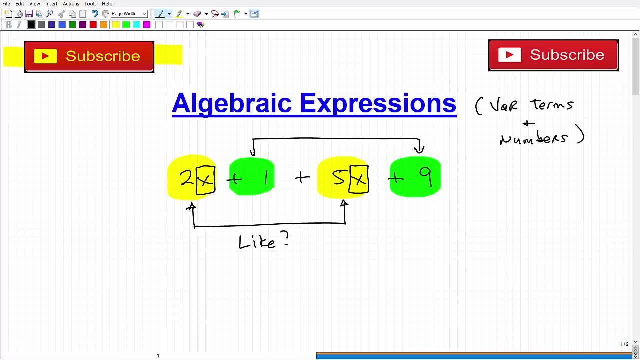 Now if an expression again doesn't have any variables, we're just talking about a numeric expression, not an algebraic expression. Okay, So now let's go ahead and combine these like terms. So 2x and 5x. let's go ahead and combine these guys. 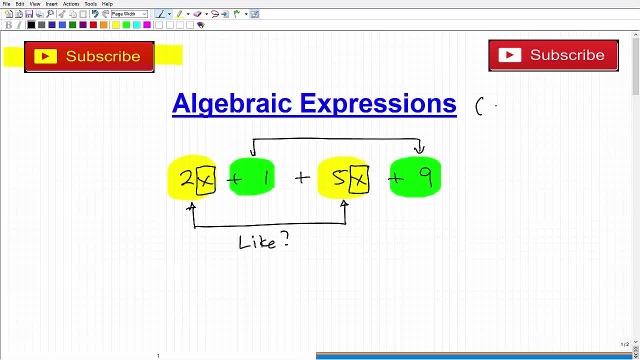 so what's going to make up an algebraic expression? are going to be variable, variable terms, right, and numbers, and these numbers can be fractions, they can be integers. positive, negative decimals doesn't make a difference right now. if an expression again doesn't have any variables, we're just talking about a 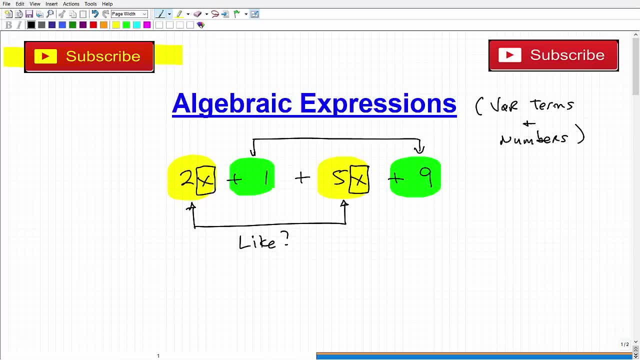 numeric expression, not an algebraic expression. so now let's go ahead and combine these like terms. so 2x and 5x, let's. let's go ahead and combine these guys, because they're alike. the variables are exactly the same. all we have to do is add the coefficients. so 2 and 5 is 7, so this is. 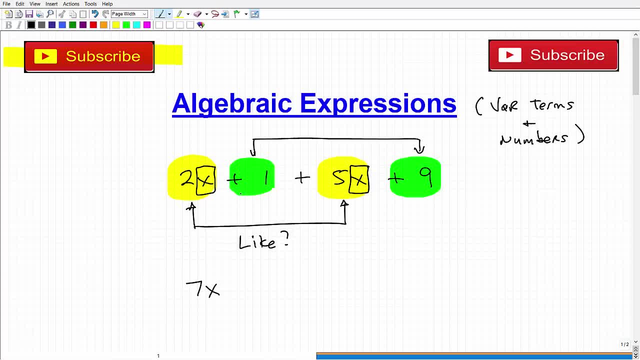 going to be 7x and then the numbers. here we have a positive 1 and a positive 9. we just add these guys together, that's going to be 10. okay, and that's it. so this is our answer, all right, so if you were to, 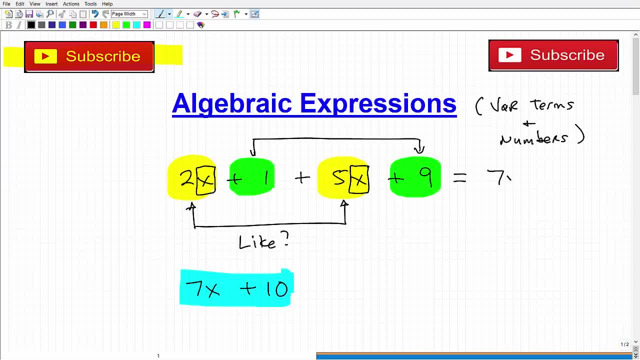 take this and simplified, our answer is 7x plus 10. all right, so this is what this is equal to. all right, now that you're saying: well, this is an equation, well, I'm just stating: this is equal to this, but you wouldn't be given this as a problem. 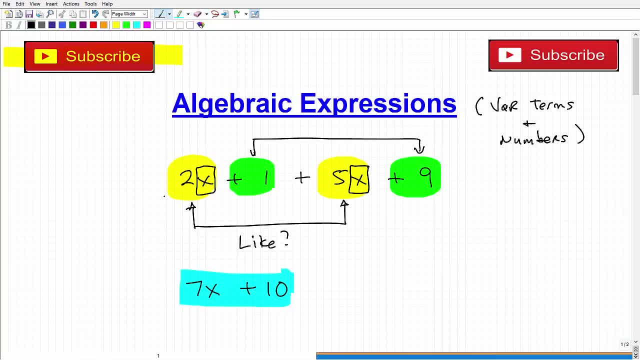 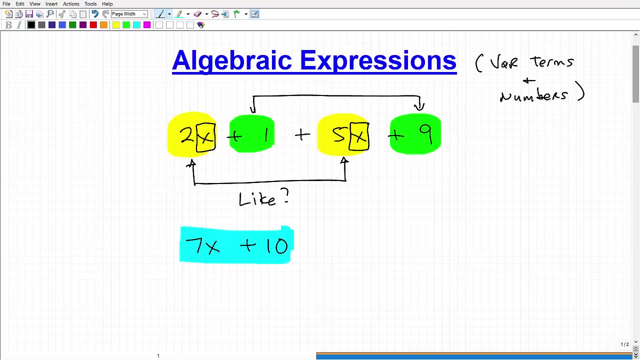 and you would be. you would be told, you know that through your directions or teachers, to simplify this algebraic expression. so real basic understanding on what that is okay. now, another thing we do with algebraic expressions is evaluate. so let's actually just use this problem here. let's scoot this guy over right there and you might be asked to evaluate. 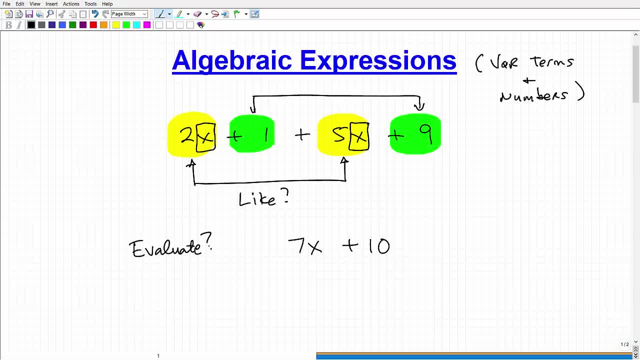 something you evaluate. so what does that mean? so to evaluate an expression, an algebraic expression, means that we're going to substitute some value in for the variable and then we're going to simplify what's left. so, for example, I could say: evaluate the algebraic expression or the 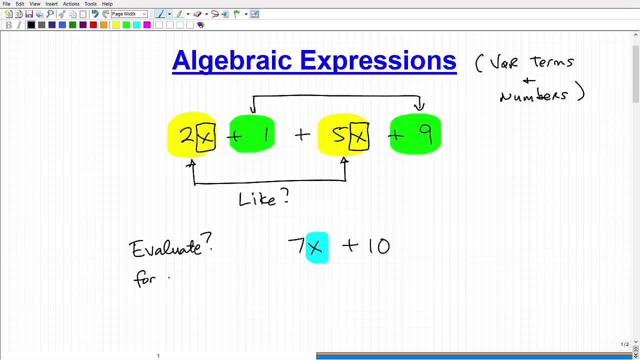 expression 7x plus 10, for X is equal to 2. okay, so what does that mean? well, it means to replace the X. okay, the variable, and you might have multiple variables here, both. so whatever variables you're going to be given values for, you're. 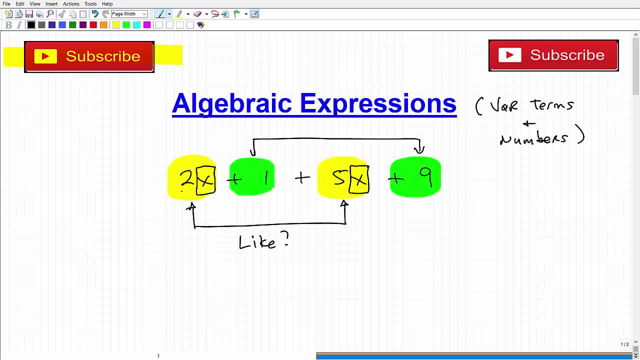 Because they're alike. the variables are exactly the same. all we have to do is add the coefficients. So 2 and 5 is 7.. So this is going to be 7x, And then the numbers. here we have a positive 1 and a positive 9.. 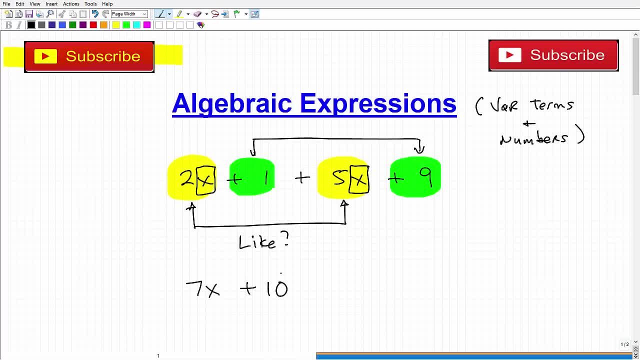 We just add these guys together, that's going to be 10.. Okay, And that's it. So this is our answer. All right, So take this and simplify it. Our answer is 7x plus 10,, all right? 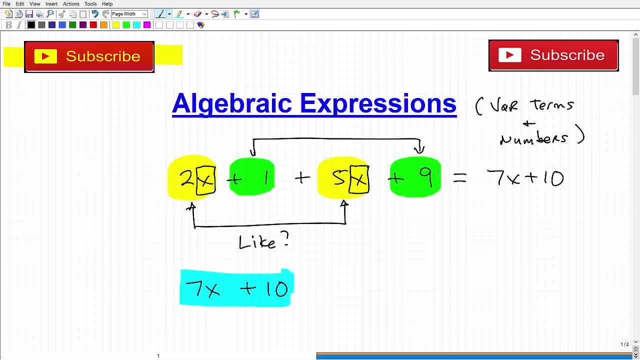 So this is what this is equal to. all right, Now you're saying: well, this is an equation. well, I'm just stating this is equal to this, But you wouldn't be given this as a problem. you would be told. you know through your 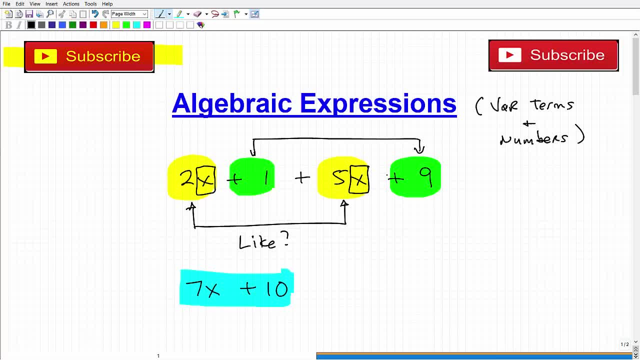 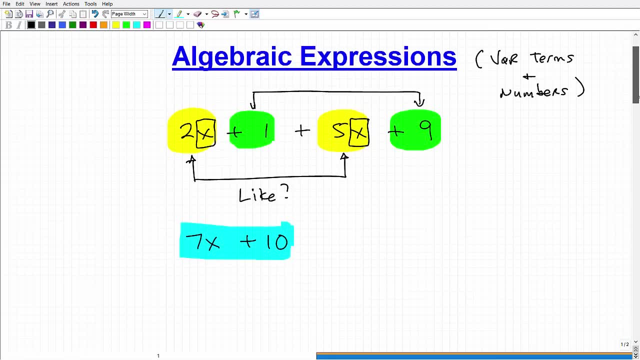 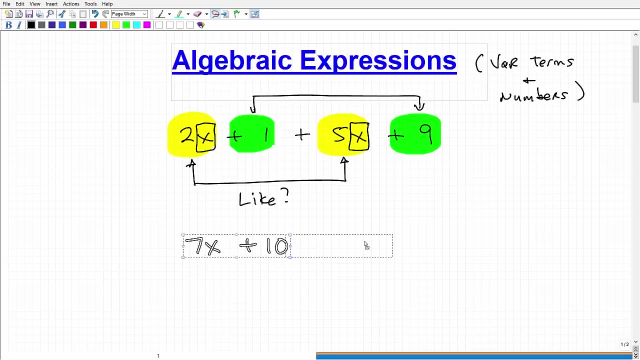 directions or teachers to simplify this algebraic expression. So real basic understanding on what that is Okay. So another thing we do with algebraic expressions is evaluate. So let's actually just use this problem here. Let's scoot this guy over right there. 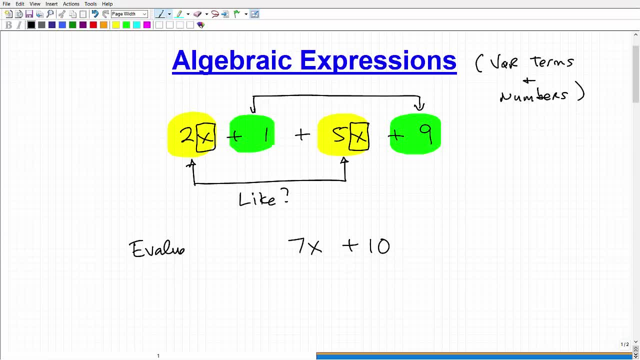 And you might be asked to evaluate something. Evaluate, So what does that mean? So to evaluate an expression, an algebraic expression, means that we're going to substitute some value in for the variable And then we're going to simplify it. 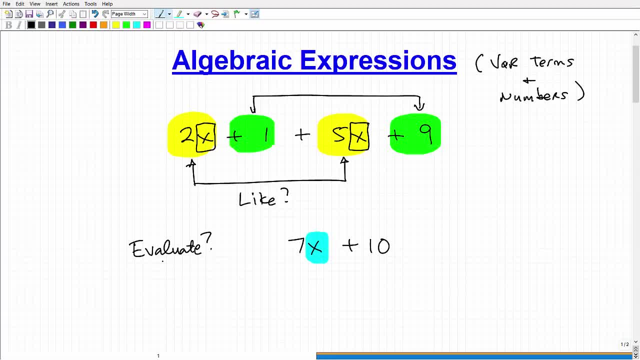 Okay, We're going to simplify what's left. So, for example, I could say: evaluate the algebraic expression, or the expression 7x plus 10, for x is equal to 2, okay, So what does that mean? Well, it means to replace the x, okay, the variable. 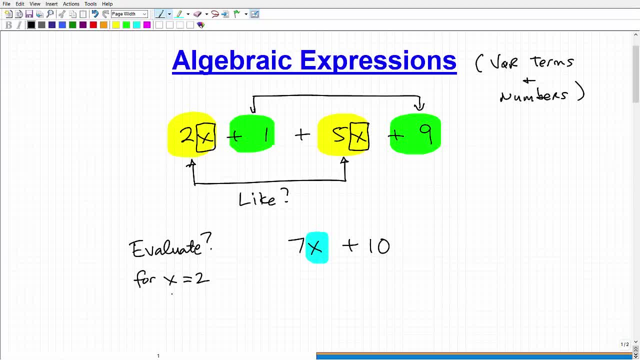 And you might have multiple variables here. So whatever variables you're going to be given values for, you're going to replace that variables with the variable. You're going to replace that variables with the actual value given. So in this case I want to know what this is equal to when x is equal to 2.. 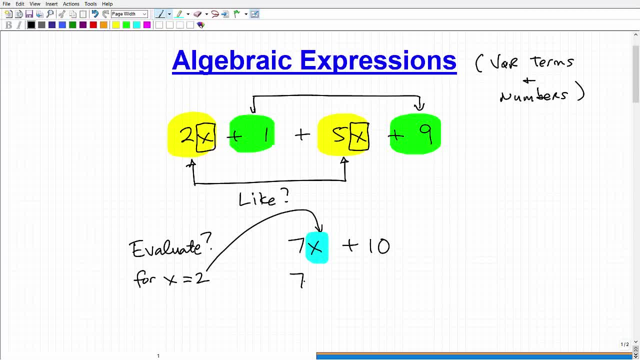 So we're going to just substitute this x for 2.. Now I want to stress something here. Let me write this out. I'm going to stress something. It's critical, critical, critical. So I need you to pay attention, all right. 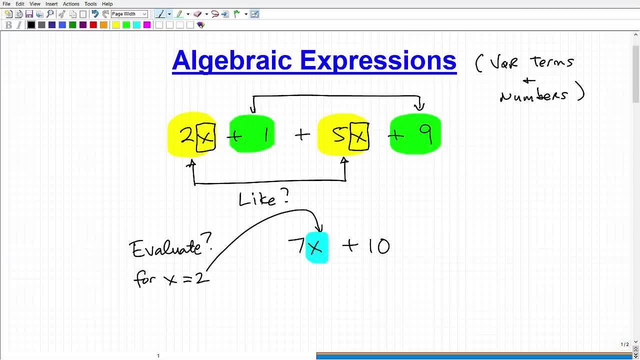 going to replace that variables with the actual value given. so in this case I want to know what this is equal to when X is equal to 2. so we're going to just substitute this X for 2. now I want to stress something here. let me write this out, that I'm going to stress something. it's critical. 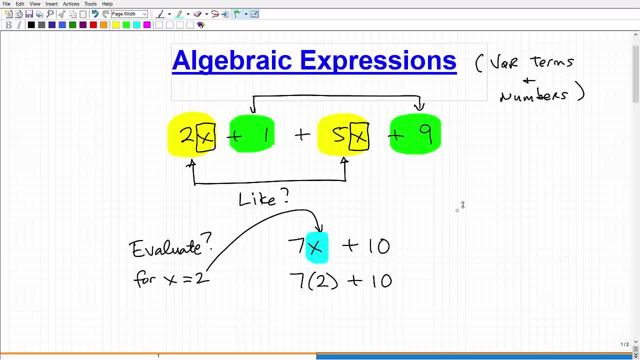 critical, critical. so I need you to pay attention. all right, so I'm going to put a big flag here. pay attention to what I'm going to say, and hopefully you've already been paying attention. but this is extremely important when you substitute a number in for a variable. 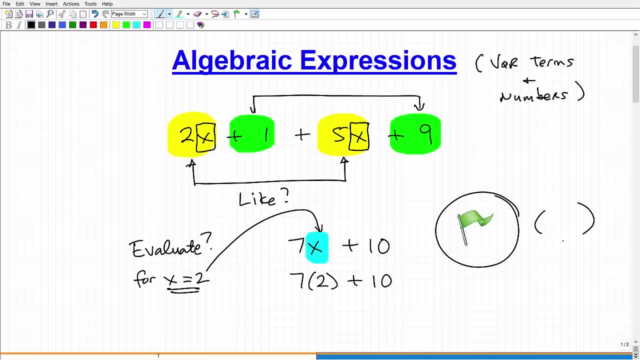 you always, always, always use parentheses around that number or that value. so, for example, you notice I put the 2 inside parentheses. parentheses here. okay, don't do this. if it's 7x plus 10 and X is equal to 2, and you're going. 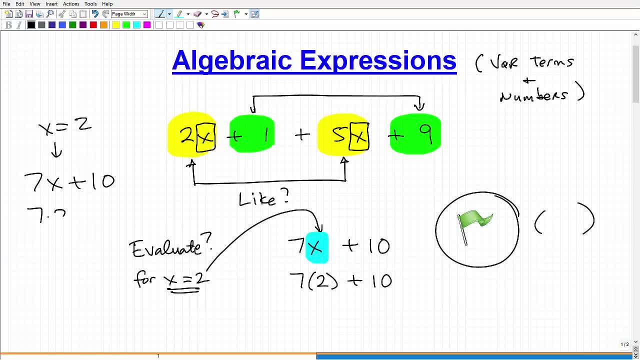 to substitute that. in so many students they do this. so 7 times 2 plus 10, that gets you in big trouble in math. okay, you must use parentheses. okay, just take it from me. I've been doing this for many years, including decades. okay, and you can. 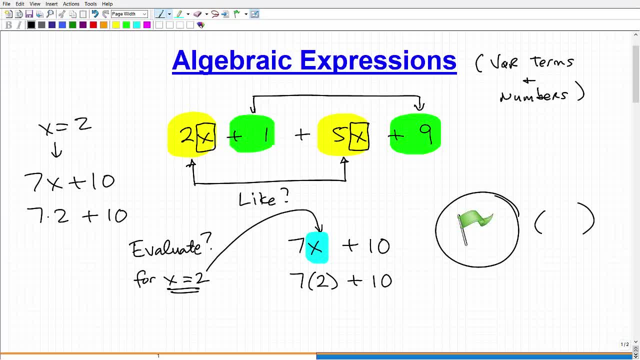 see where students mess up. you don't want to do that. get in the habit of using parentheses now. once you've done that, we need to then simplify this remaining numeric expression and we just use the order of operations. so it's really important that you understand the order of operations when you're dealing. 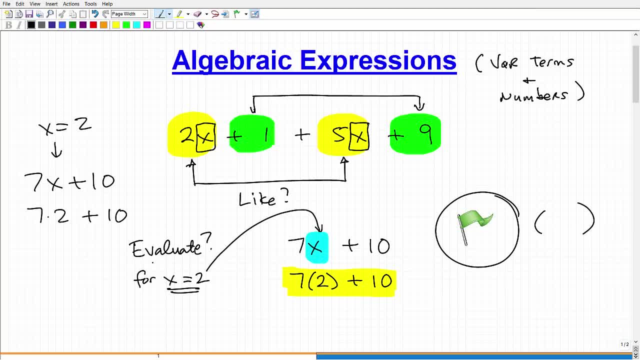 with these expressions. okay, because oftentimes you'll be asked to evaluate an algebraic expression, turning it into a numeric expression, and then you're going to have to use your arithmetic skills, your knowledge of fractions, positive, negative numbers, order of operations, etc. to simplify this down now. this is extremely easy problem to do. it's very basic, right. 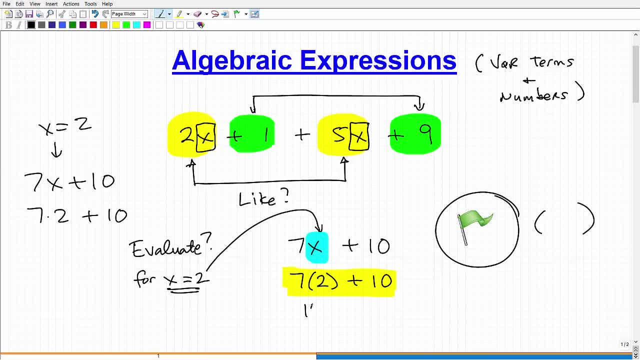 so 7 times 2. I'm going to do multiplication before addition. this is gonna be what? 14 plus 10? so my answer is 24. so I'm done. but you know these problems can get much more sophisticated if you will. you know more variables, or they're asking to evaluate the fractions of decimals. so 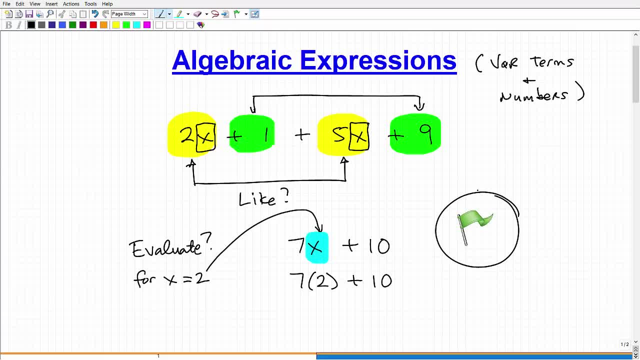 So I'm going to put a big flag here. Pay attention to what I'm going to say, And hopefully you've already been paying attention, but this is extremely important. Okay, When you substitute a number in for a variable, you always, always, always use parentheses. 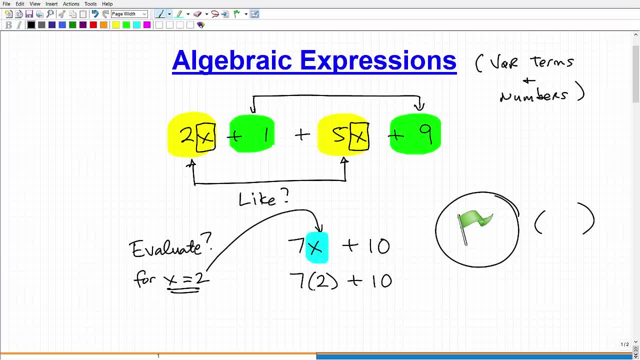 around that number or that value. So, for example- notice I put the 2 inside parentheses here- okay, Don't do this. If it's 7x plus 10 and x is equal to 2 and you're going to substitute that in so many. 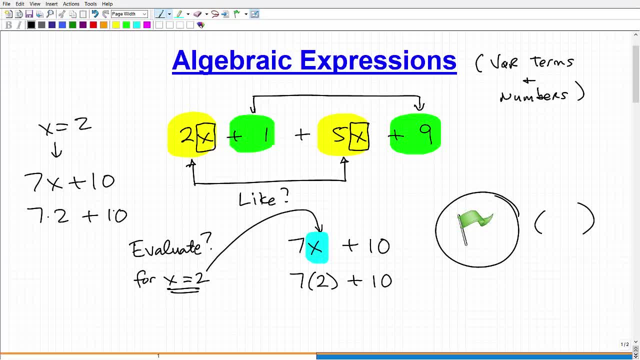 students. they do this: oh, 7 times 2 plus 10.. That gets you in big trouble in math. Okay, Don't use parentheses. okay, Just take it from me. I've been doing this for many years, including decades, okay. 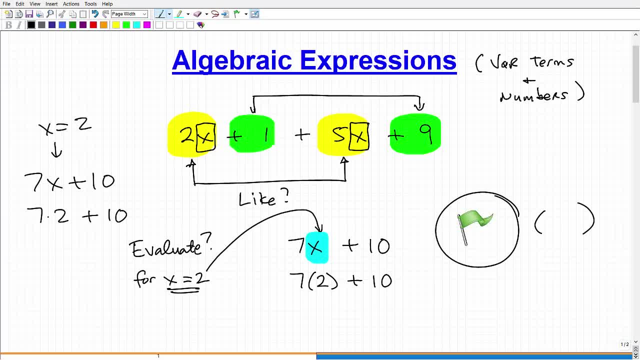 And you can see where students mess up. You don't want to do that. Get in the habit of using parentheses Now. once you've done that, we need to then simplify this remaining numeric expression and we just use the order of operations. 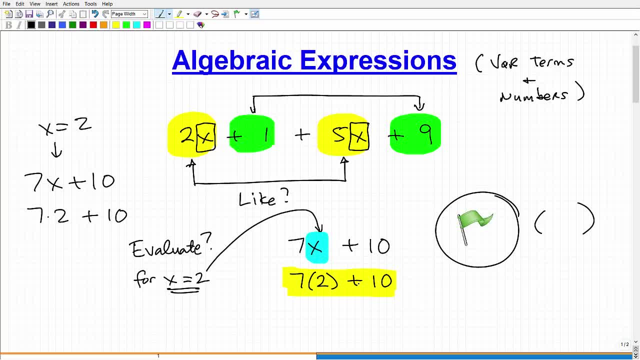 So it's really important that you understand the order of operations when you're dealing with these expressions. okay, Because oftentimes you'll be asked to evaluate an algebraic expression, turning it into a numeric expression, and then you're going to have to use your arithmetic skills, your 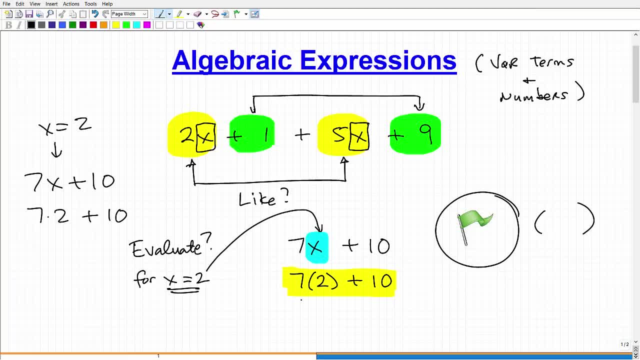 knowledge of fractions, positive and negative numbers, order of operations, etc. to simplify this down Now, this is an extremely easy problem to do. It's very basic, right. So 7 times 2,- I'm going to do multiplication before addition. 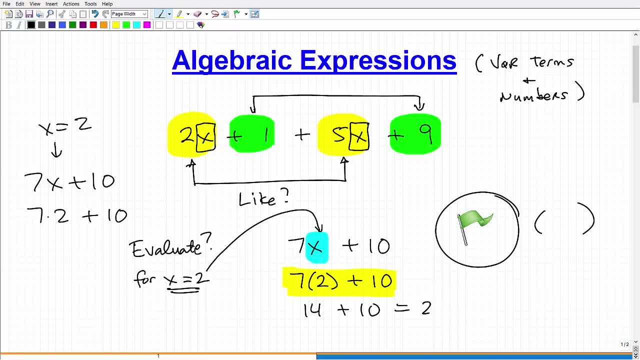 This is going to be what? 14 plus 10.. So my answer is 24.. So I'm done. But these problems can get much more sophisticated, if you will: more variables, where they're asking you to evaluate fractions and decimals. 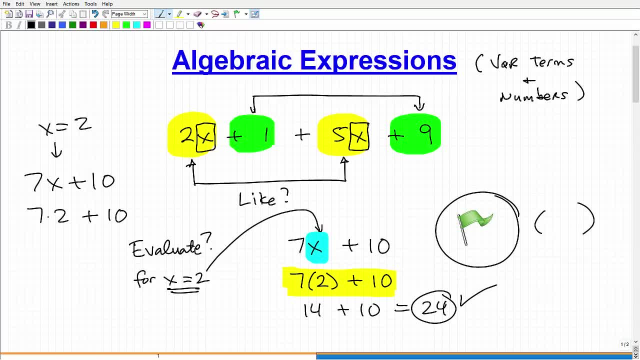 So you have to practice this stuff. But what I find with students is, if you don't understand the basic, the basic idea behind the concept, then you're going to likely struggle. So hopefully in this video we broke down what an algebraic expression is.